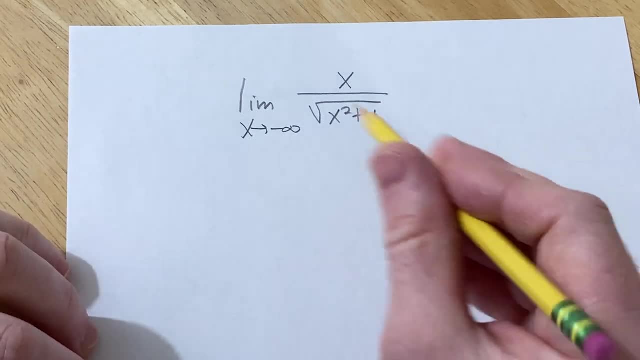 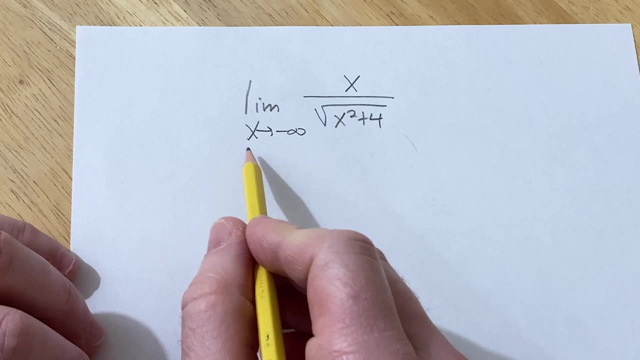 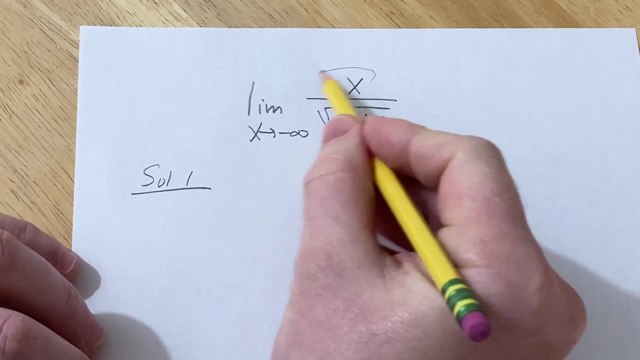 Hello, in this problem we are going to find the limit as x approaches- negative infinity of x over the square root of x squared plus 4.. So to do this, we are going to do it two different ways. So solution one: we're going to use intuition. I'm just going to go ahead and 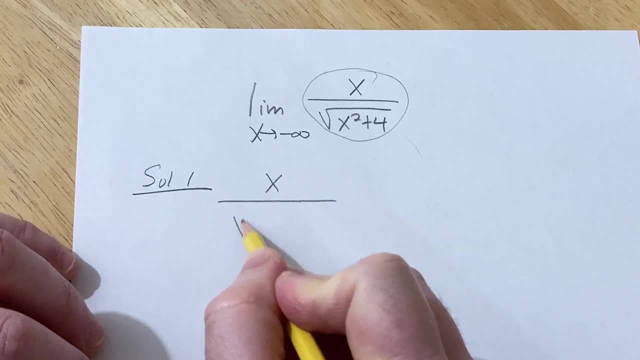 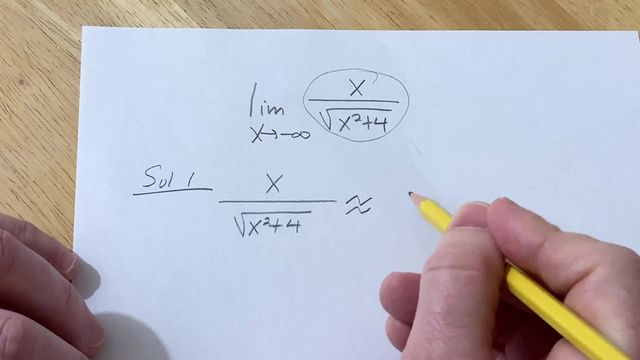 write this down. So this is x over the square root of x squared plus 4.. So when x is approaching negative infinity, x squared is going to be positive and really, really huge. So the 4 doesn't really matter. So this is approximately equal to x over the square root of x squared. 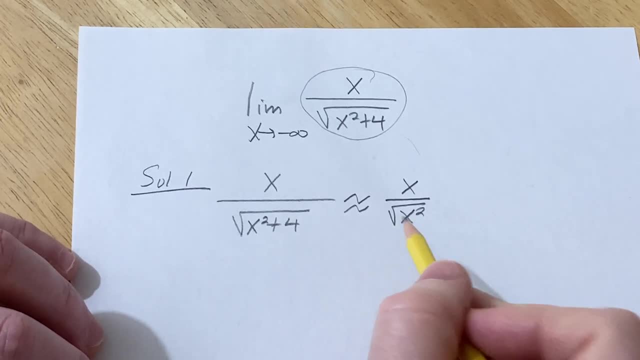 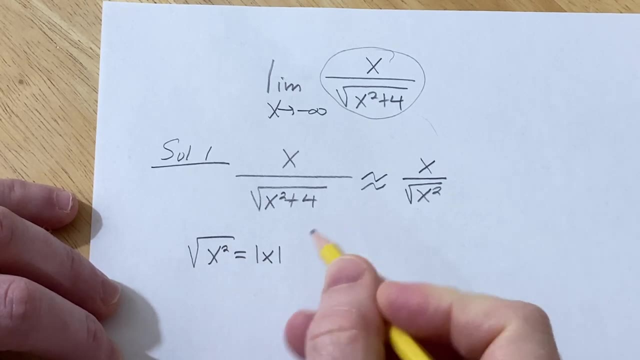 because we can drop the 4.. Now, the square root of x squared is actually something that we need to know. It's the absolute value of x and that's a piecewise function. So that's x if x is greater than or equal to 0.. 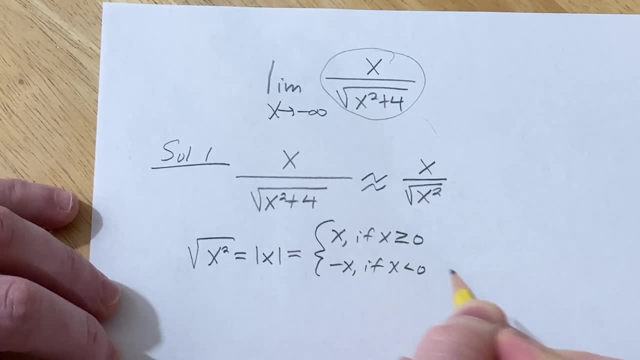 And it's minus x if x is less than 0.. So in this particular problem, since x is approaching negative infinity, that means that x is less than 0. So that means that the square root of x squared, which is the absolute value of x- we use this condition here- it's equal. 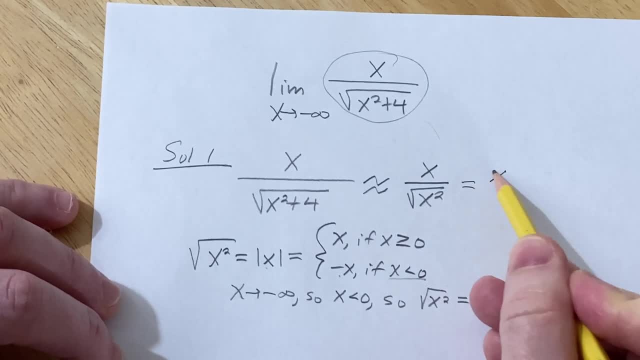 to negative x. So this here is actually equal to x over negative x. These cancel and you just get negative 1. And that's going to be the limit. So that's really the key right here. This is the key to doing this problem. Let me show you another way to do it. Solution. 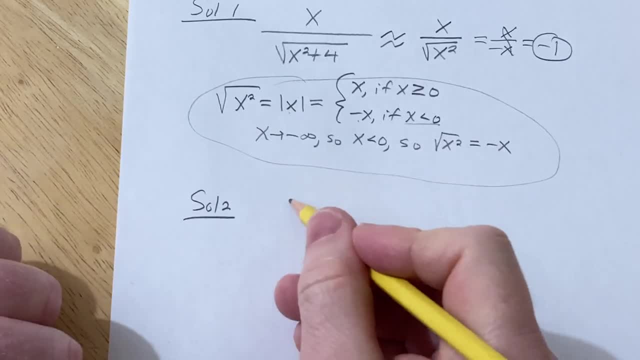 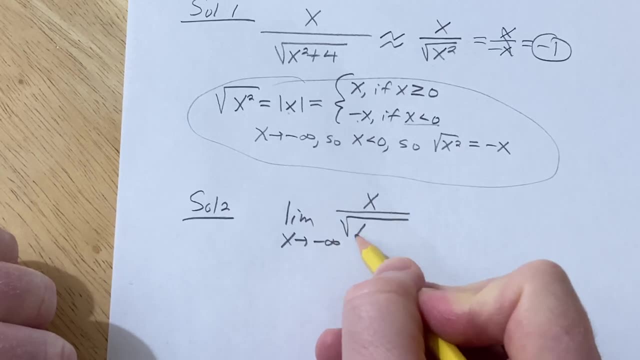 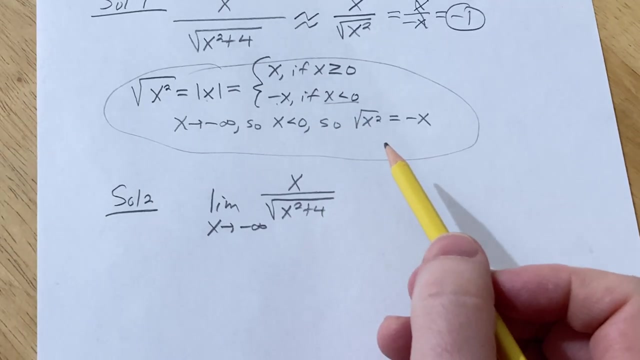 2.. Perhaps a better way to do it, a better way to show work, is the following: So we take the limit as x approaches negative infinity of x over the square root of x squared plus 4.. So we can do this using this same idea, but we can be a little bit more precise with. 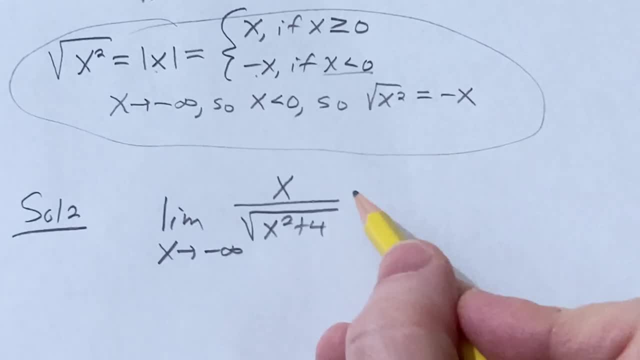 our work here. So what we're going to do now is we're going to basically multiply by 1 in a clever way. So here I'm going to multiply by 1 over negative x, And here I'm going to multiply by 1 over. 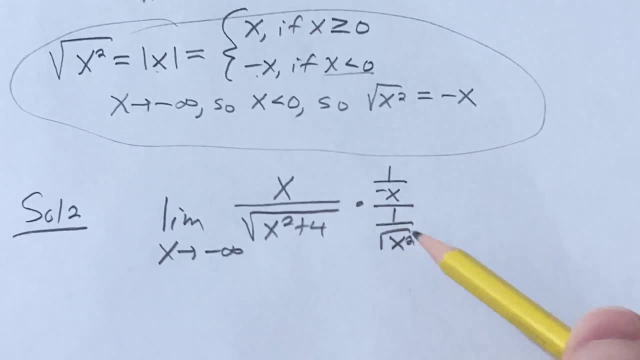 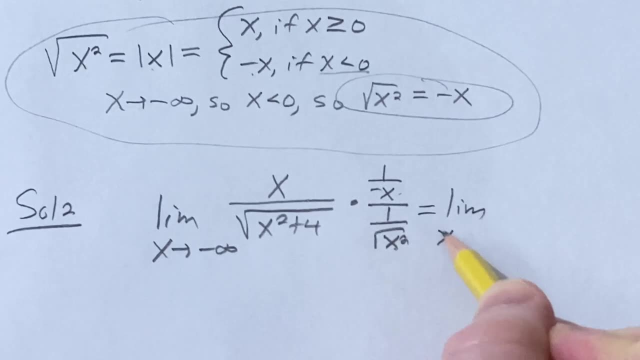 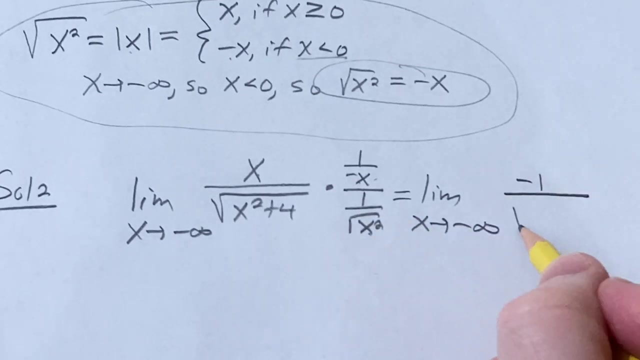 the square root of x squared. Realize that these are the same, because the square root of x squared is equal to negative x by what's written here. So this becomes the limit As x approaches negative infinity. x over negative x is negative 1. And then here we can combine.